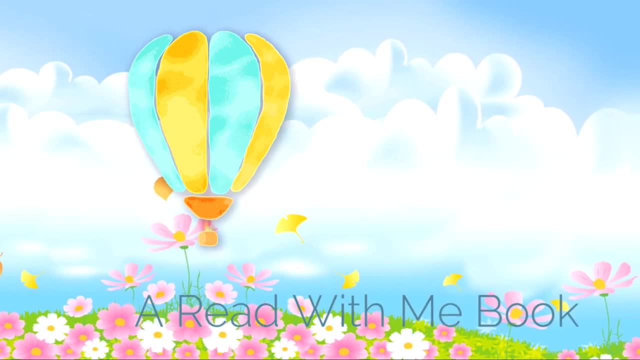 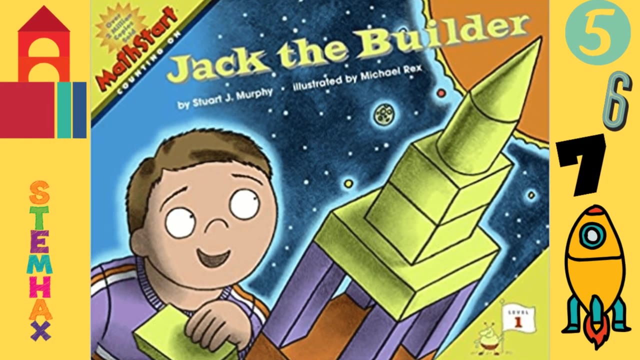 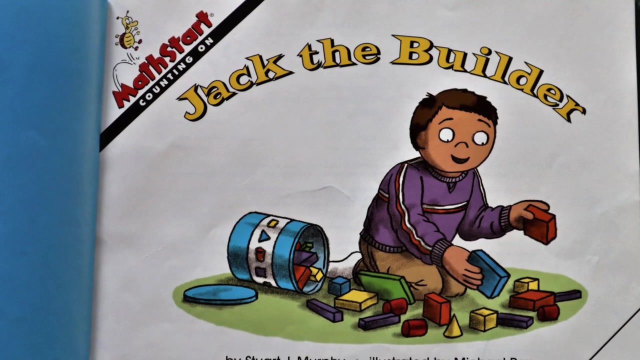 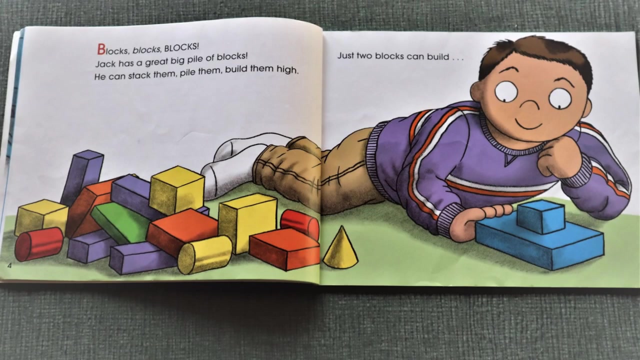 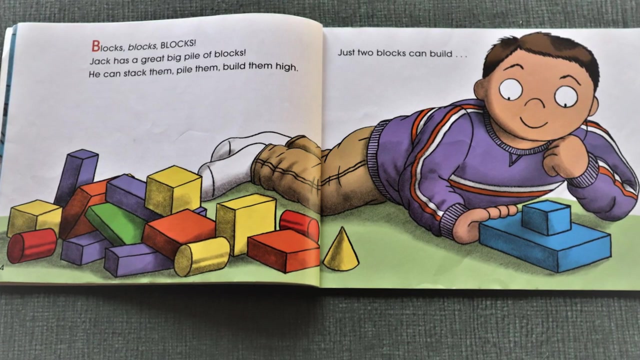 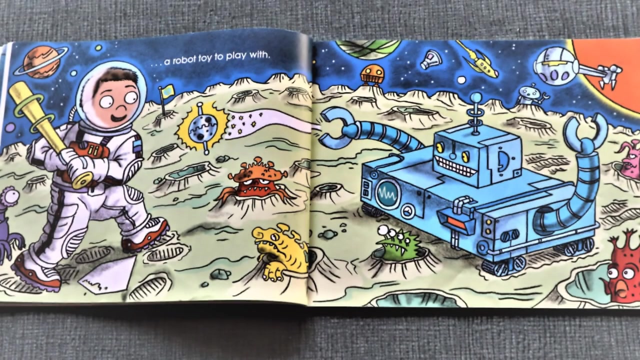 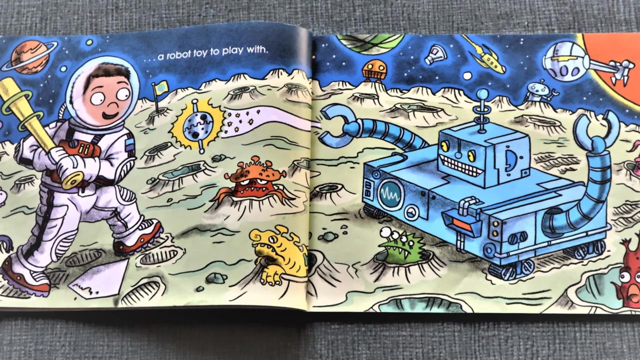 Jack the Builder by Stuart J Murphy, illustrated by Michael Rex, published by HarperCollins Blocks, blocks, blocks. Jack has a great big pile of blocks. He can stack them, pile them, build them high. Just two blocks can build a robot toy to play with. 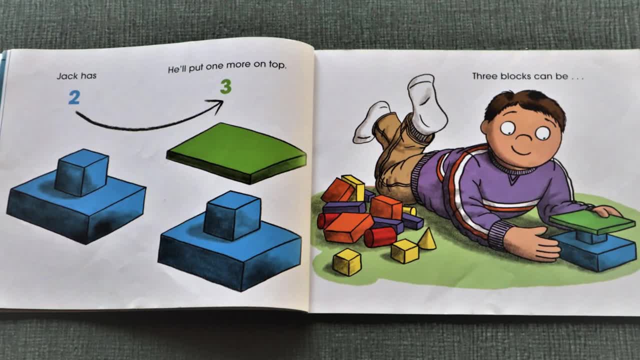 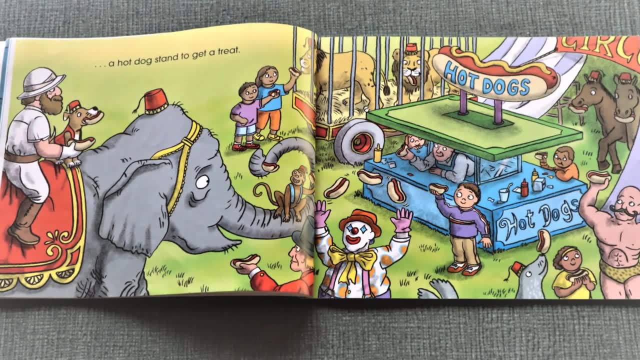 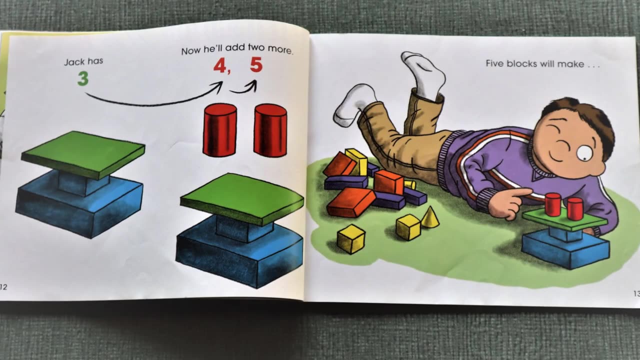 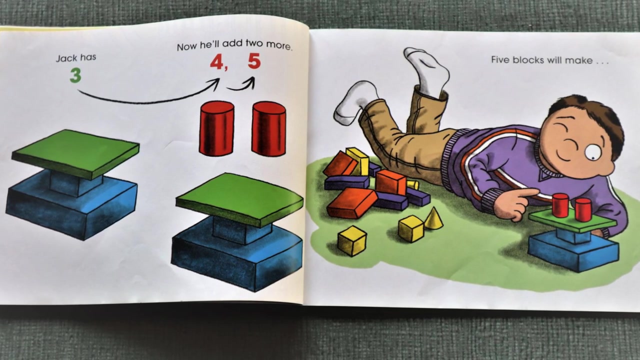 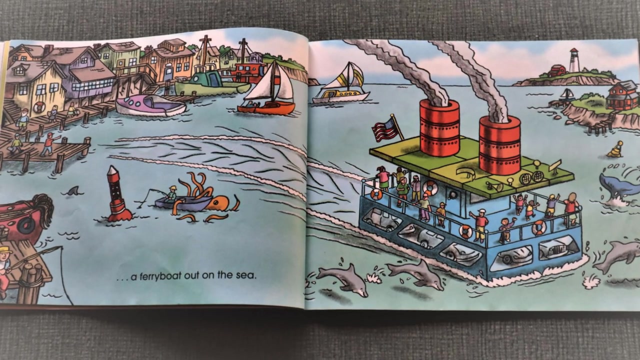 Jack has two, He'll put one more on top. Two, three, Three blocks can be a hot dog. stand to get a treat. Jack has three. Now he'll add two more. Three, four, five, Five blocks will make a ferry boat out on the sea. 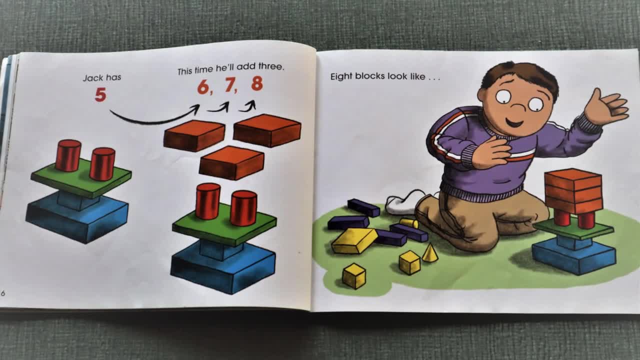 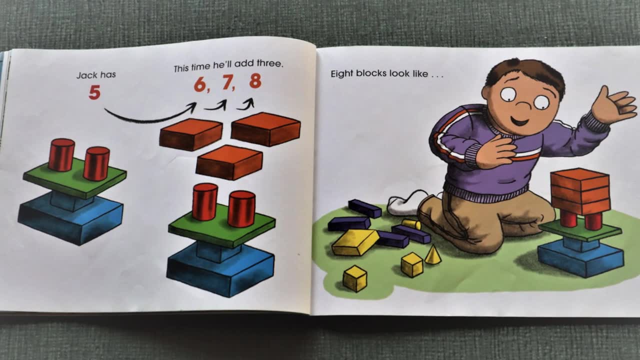 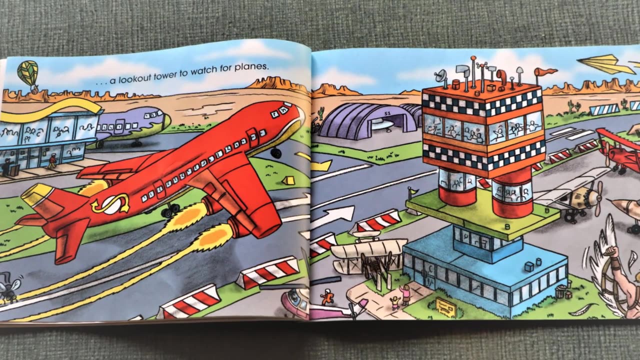 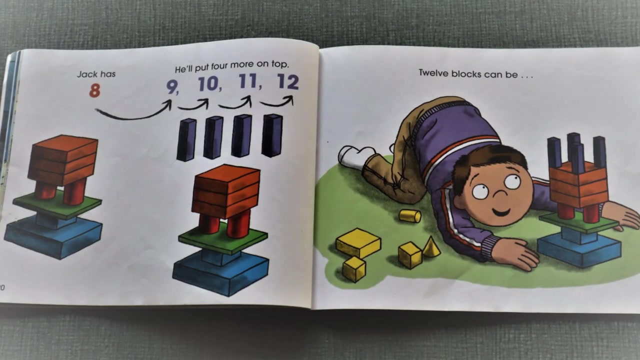 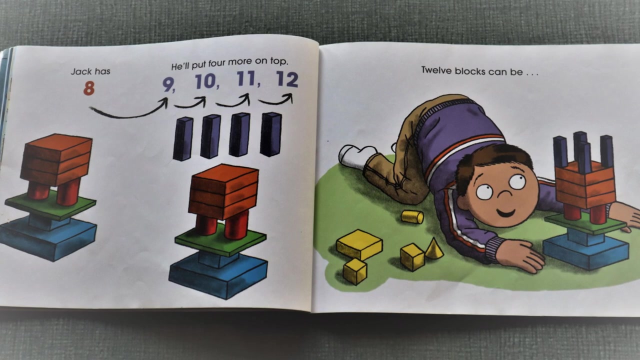 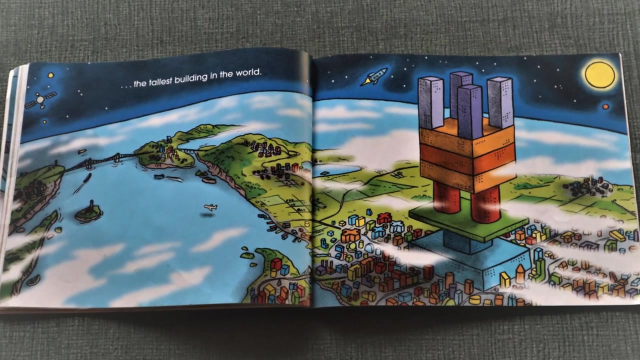 Jack has five. This time he'll add three. Five, six, seven, eight, Eight blocks look like a lookout tower to watch for planes. Jack has eight. He'll put four more on top. Eight, nine, ten, eleven, twelve, Twelve blocks can be the tallest building in the world. 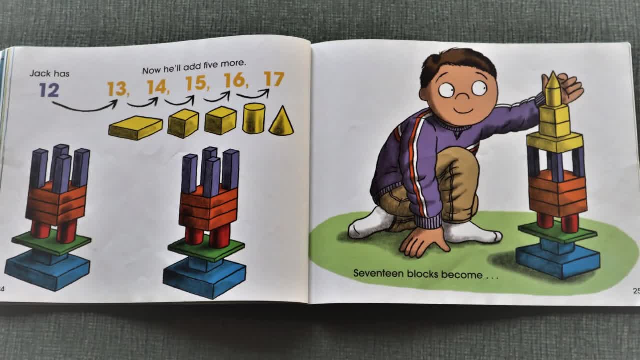 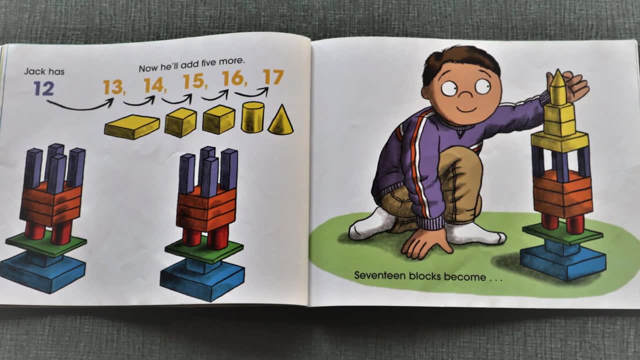 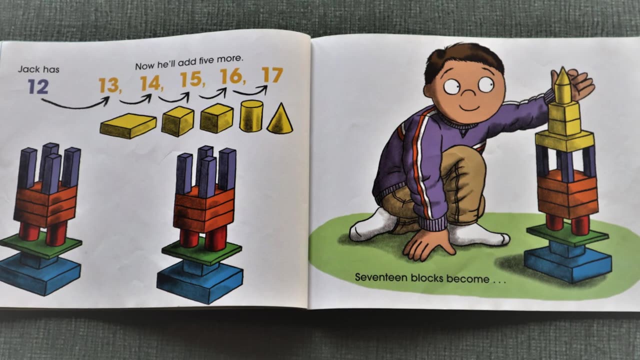 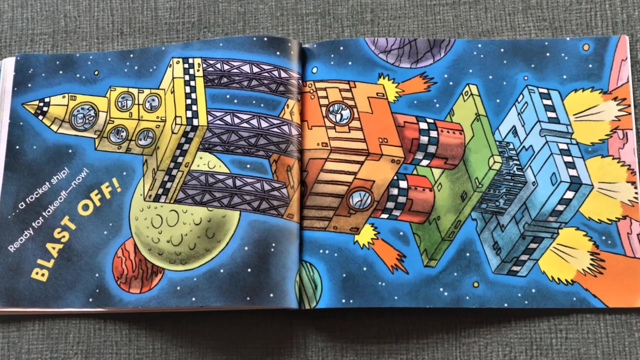 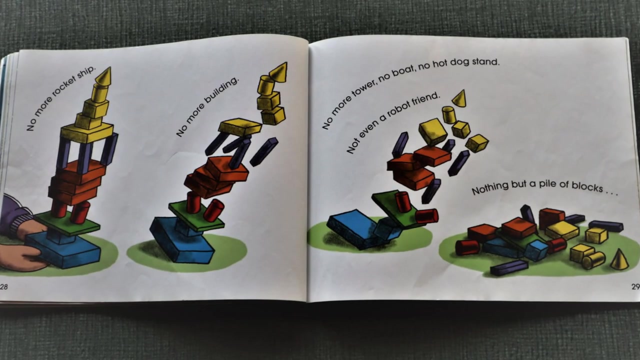 Jack has twelve, Now he'll add five more, Twelve, thirteen, fourteen, fifteen, sixteen, seventeen, Seventeen blocks become a rocket ship, Ready for takeoff. Now Blast off. No more rocket ship, No more building, No more tower, No boat, No hot dog stand.